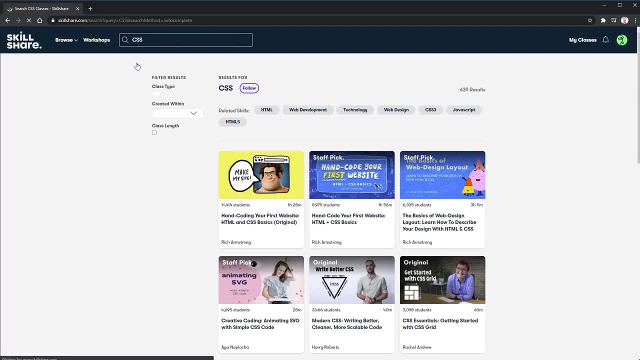 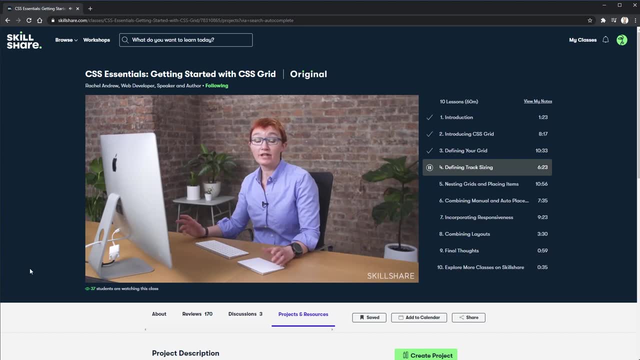 literally millions of people. It's a really awesome platform with incredible content, including getting started with CSS grid by none other than Rachel Andrew. So if grid is something you wanted to learn, you find it as a little bit confusing. You're not sure where to get started with it. 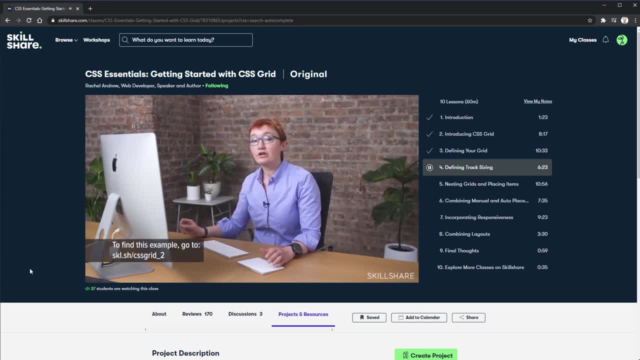 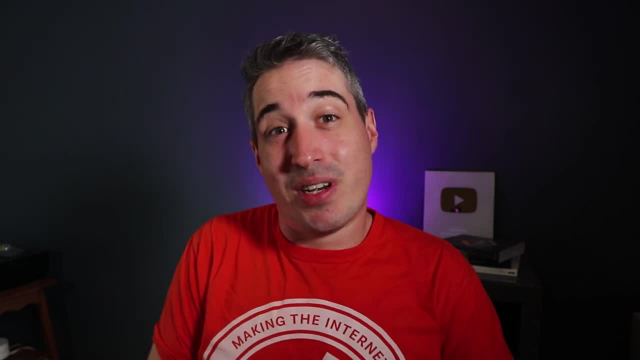 There is probably no one else you'd want to start learning grid from then, somebody like Rachel Andrew, who helped spearhead the whole getting grid to be a thing. So I mean, you can't ask for better than that If this sounds interesting to you. 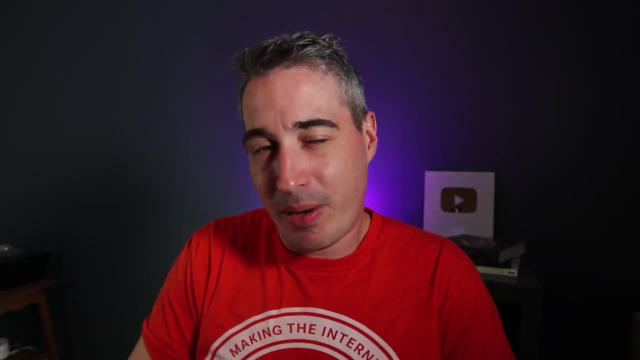 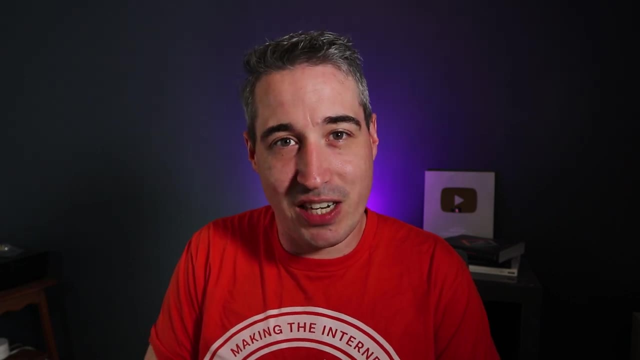 make sure you go and click the link down in the description below. The first 1000 of my subscribers who click on that link will get a two month free trial of their premium membership. Thank you very much to Skillshare for sponsoring this video. 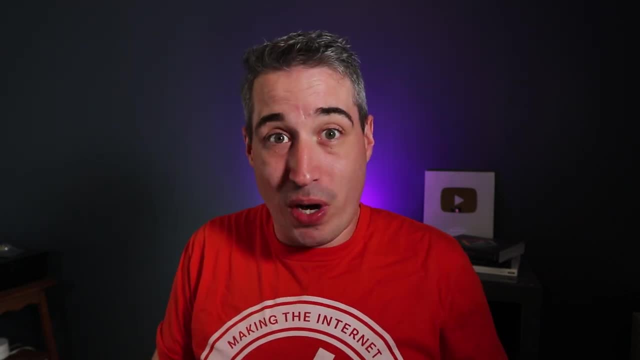 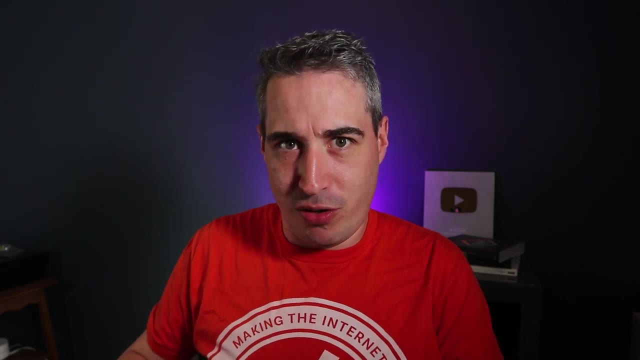 Now let's go talk about some lazy loading. So we're going to look at first is what is lazy loading, And we talked a little bit about why you should care about it already. It's all about performance, but it's all about making images that the user hasn't scrolled down to yet. 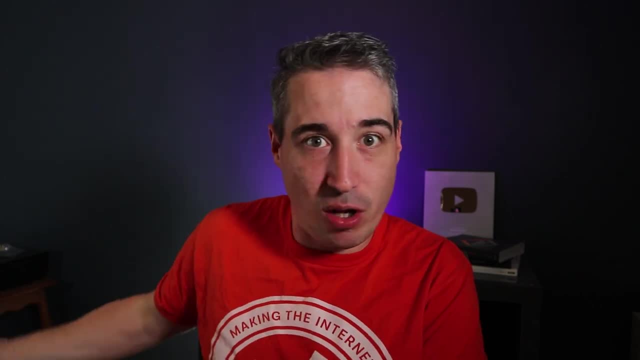 They don't load because you know if a user hasn't scrolled, they don't load There. we don't need all these things loading in for nothing. It's not only for images either. It is for iframes as well, And iframes are notorious for being really slow. 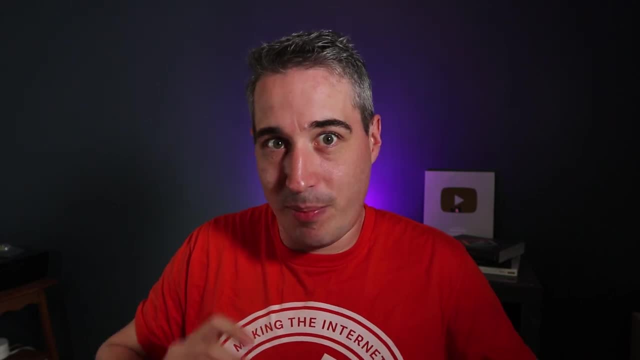 So for both of these things you can just help that first paint of your page come in much, much faster and be fully loaded. So here we are, in vs code and you can see I've brought in a whole bunch of images here. Um. 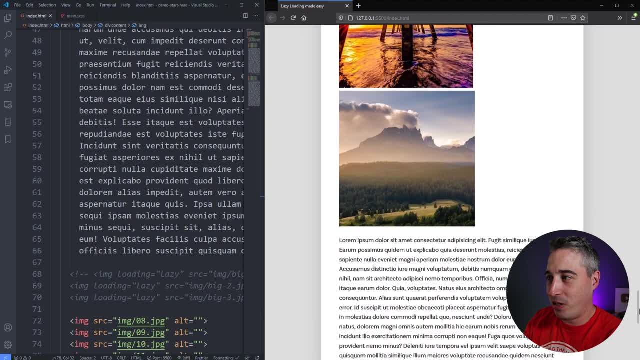 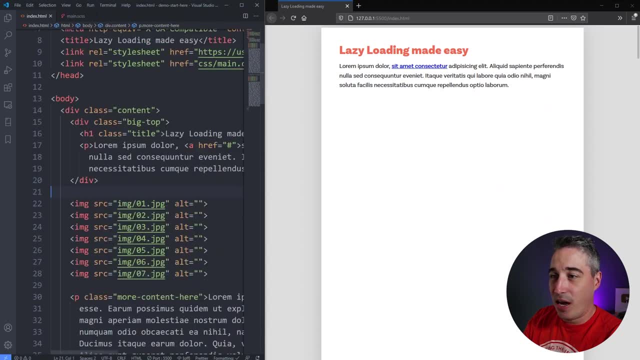 and I've made this really long page and it's really just like a demo page. a whole bunch of images that are all stacked on top and tons of filler text. Um, and I'm bringing this in just to show you really how um. 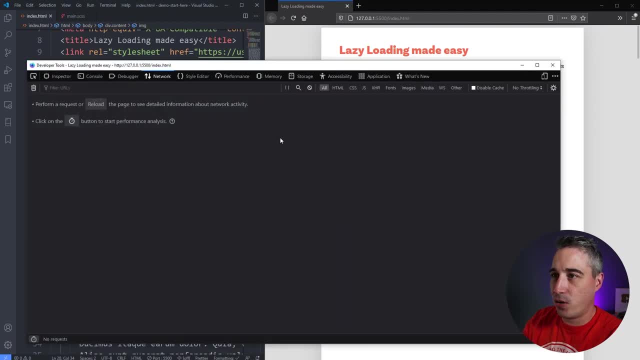 you know the power of of lazy loading. So the first thing I'm gonna do is open up my console and we can see I'm already on my network tab here. So if you're on inspector and I am in Firefox, but if you're in Chrome, 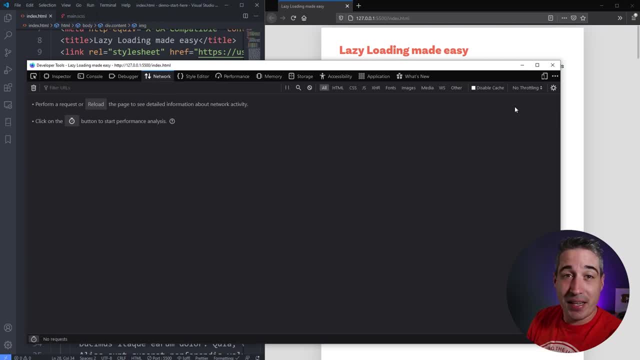 it's exactly the same. I'm sure Safari has something like this as well, And one of the nice things with this network tab is I'm going to disable cache, So it's if somebody is the first time they're on their site or their cash has been. 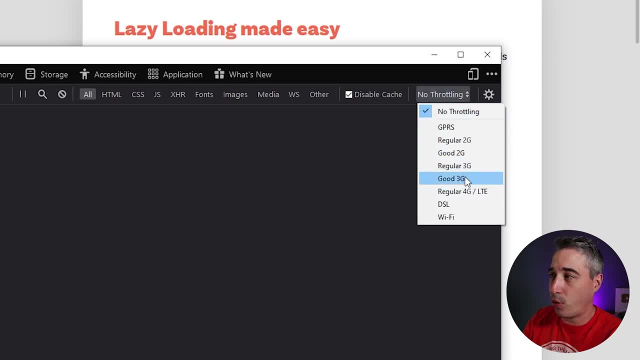 cleared for some reason and you can simulate different types of connections that people are on. So we always develop locally. things load. You could have like a five make image and it's going to load instantly because you're local on your machine. That's not. 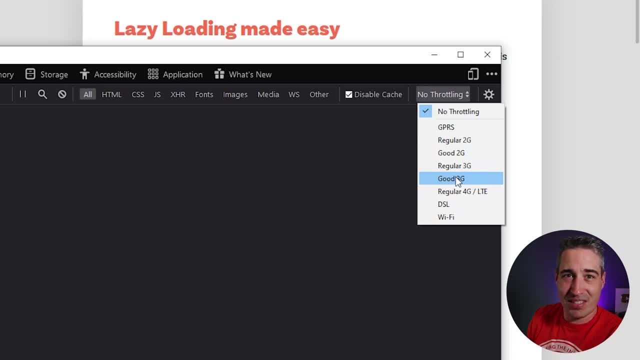 that's not realistic to the real world. Um, we're also. a lot of us developers were on state of the art devices all the time. That's not realistic. always to the real world, You had bad connections for whatever reason, even if it's a bad wifi connection. 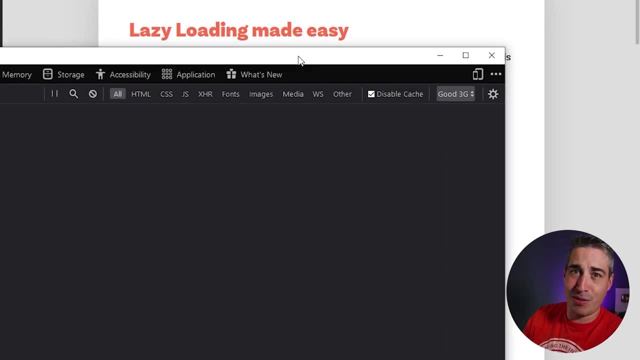 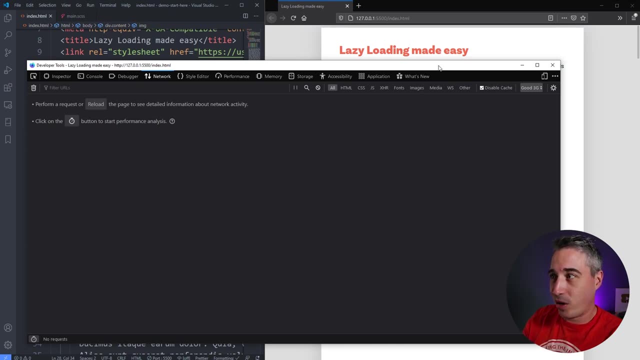 Um, so let's go to a good three G connection and I know everyone's like: Oh, we're on four G. now five G is coming. Not everyone in the world is on that. You're on old devices. There could be a number of reasons why things are slower. 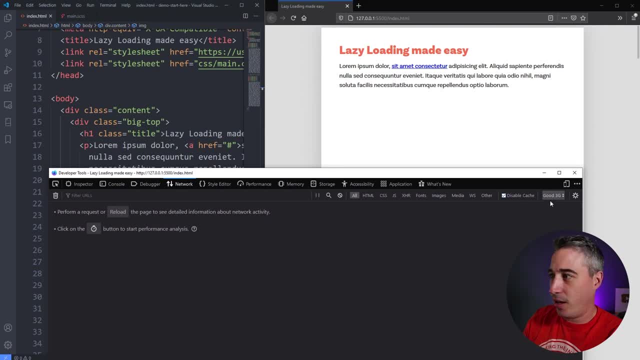 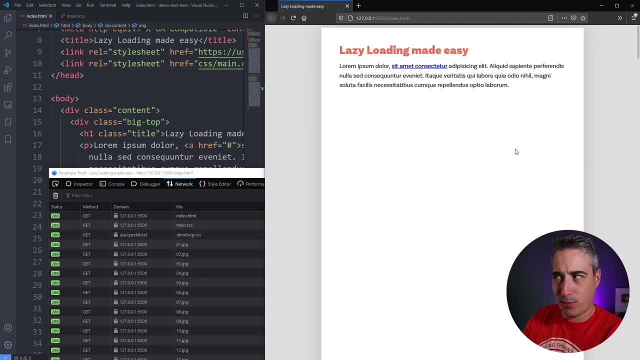 So let's simulate what it is. So by doing disable cash, good, uh, three G. I'm going to refresh my page And you can see there's some stuff going on here. We're not going to worry, but you can actually see how the page took some time to load in there. 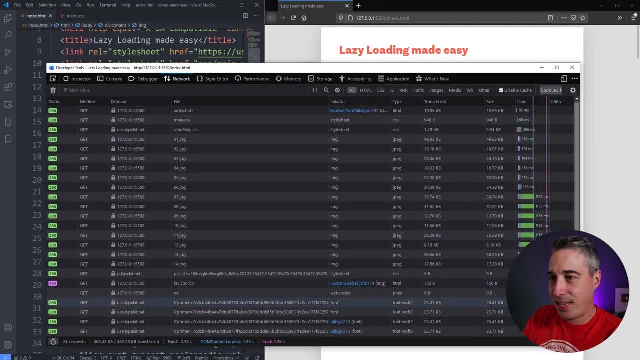 Um, and what's happening with this network tab is you can actually see how long everything's taking to load in. So you can see that it first took 96 milliseconds. here You can see nothing was really taking too long. Oh, I have type kit. 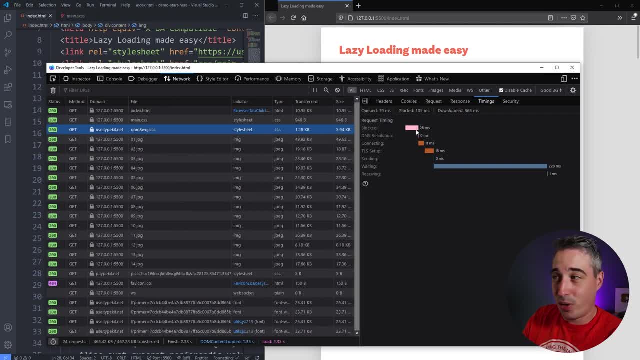 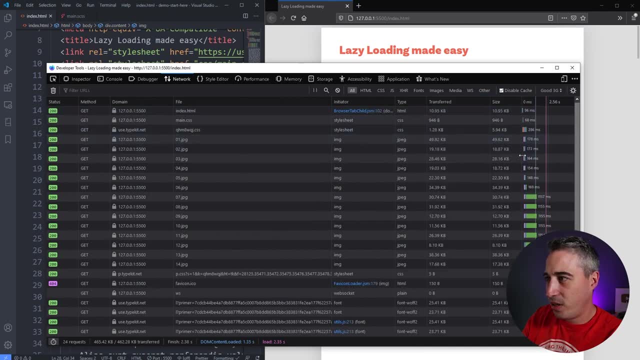 So that's slowed things down slightly. Um, it blocked the site from loading for 26 seconds and then it had to wait a little while before finally it got what it needed. But where did things really slow down over here? We had some images that were coming in. 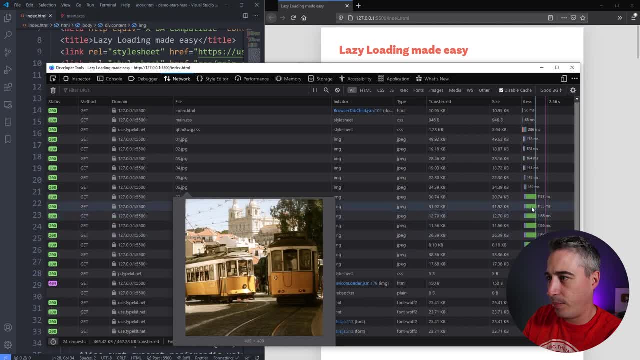 And then, Oh well, look at this Some of these images. they took a long time to come in, My goodness, And they're not even big images like 49 KB, 19 KB, Some of these ones that took a lot longer. 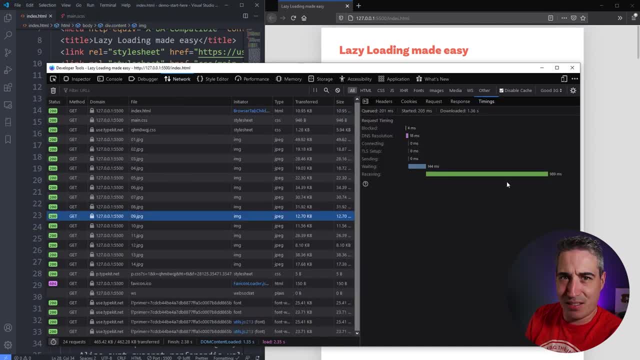 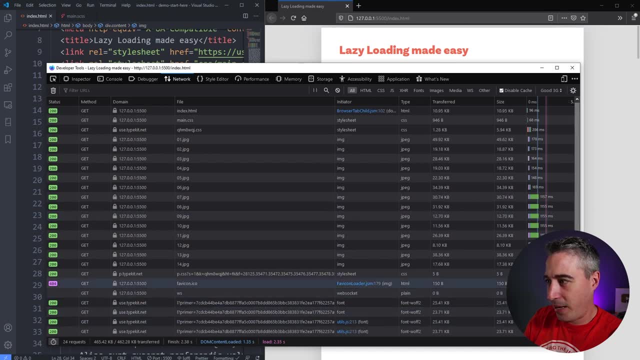 there are like 12 KB, but it took a long time to receive this because it's a slower internet connection. Huh, That's interesting, right, And so all these were coming in. you can see it took a while for the page to finish. 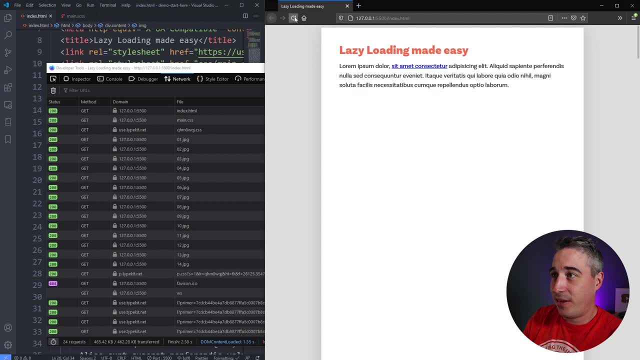 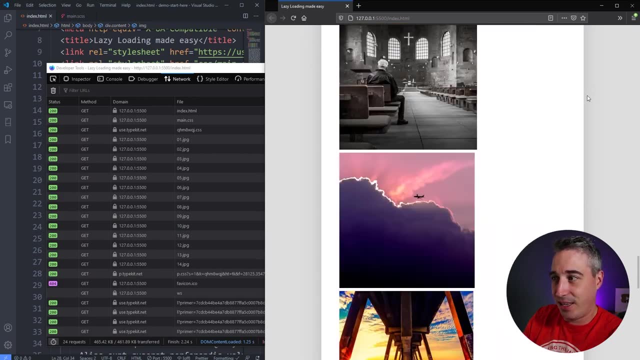 uh, coming all the way in to get to that last image. So, and again, let's just hit refresh and see. it takes a little while for that to come in And then, and obviously, all this is, everything is in there now. 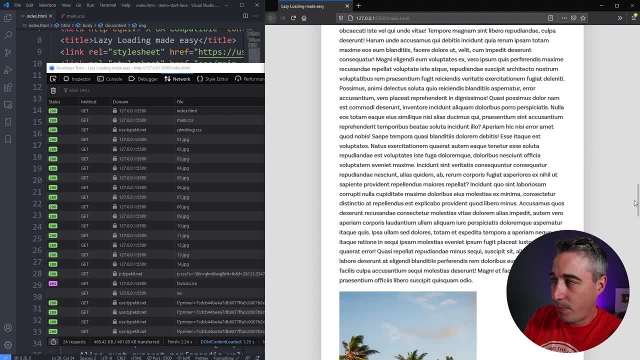 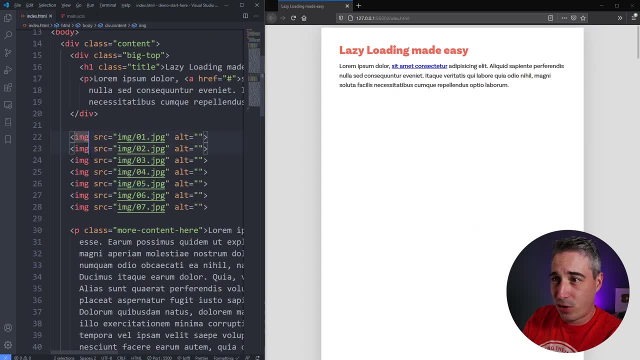 but these images are tiny images, right? Um? but before we we look at what happens with bigger images, I want to show you how easy this is now because, as I said, you could do this with JavaScript. Uh, I'm just going to go there. 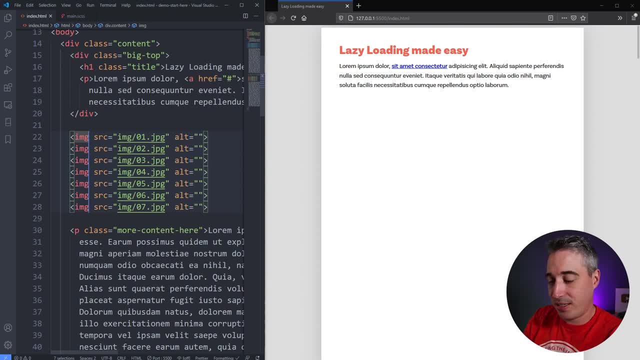 If you don't know about this, in VS code you can place your cursor in multiple places at once, So I'm just holding down alt while I do that, Cause I am on windows. I'm guessing it's option on a Mac, but I could be wrong on that one. 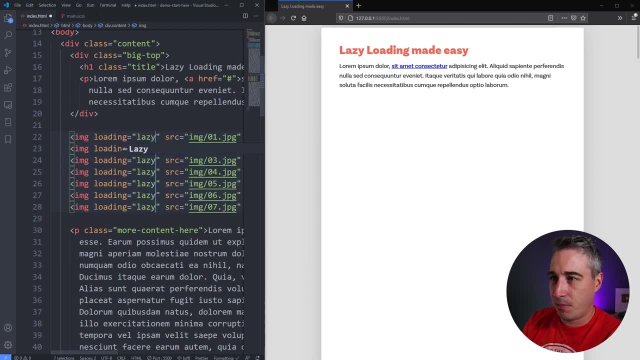 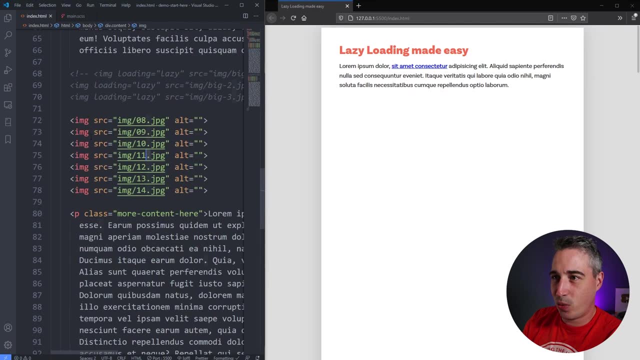 Um, so what I'm in right now is loading is equal to lazy, nice and easy Right And let's hit save and whoops, I forgot Let's. uh, I wanted to do that down here as well, So let's come down here and do it on these ones as well. 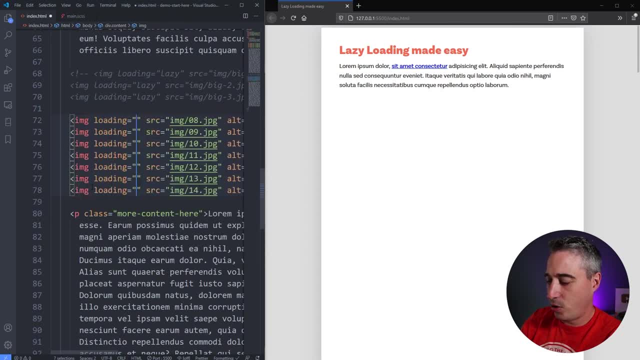 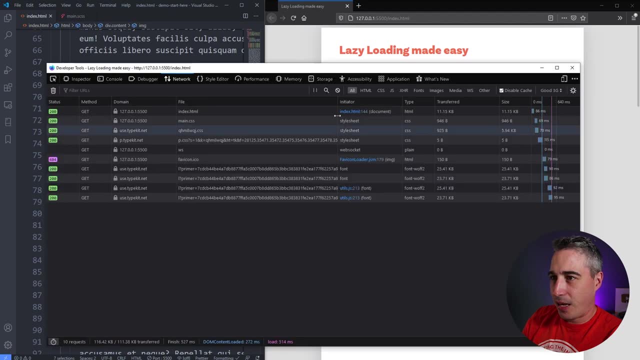 Could have done that all at once, but that's all right. Loading is equal to lazy and we'll hit save. Now let's open that network tab back up again And you'll notice there's a lot less stuff in here. Where's? where's the images that haven't loaded in? 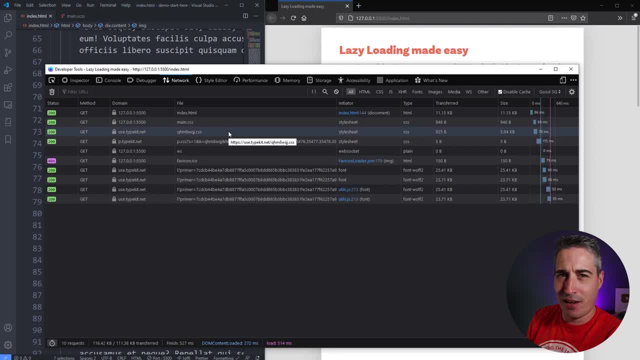 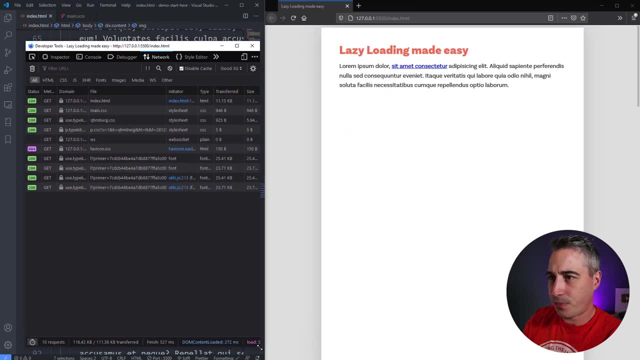 There's been no network requests for those images. That is interesting, Right, And now, uh, I want to leave this up here. Let's just shrink this down a little bit on the side here, Um, like that, So we can see as I scroll here and before we get to the. 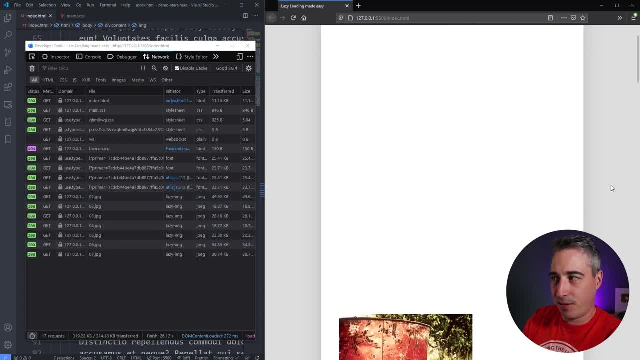 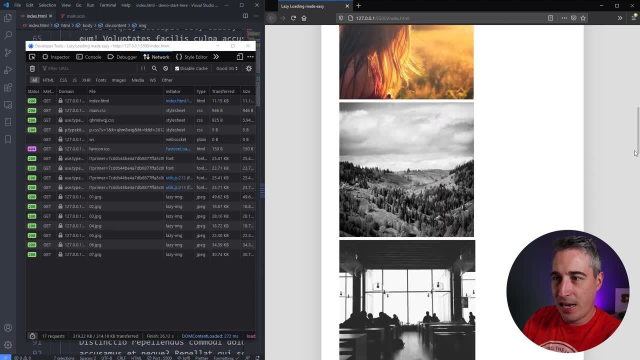 images are right. as the images came in, you can see boom. all of those came in and but it's only stopped at image number seven, because then I had that wall of text. So now I'm going to keep going And then as we approach, 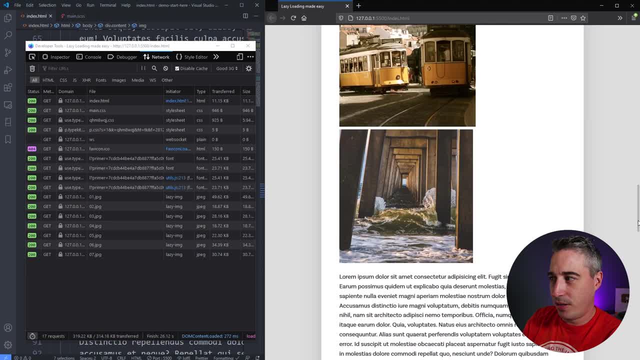 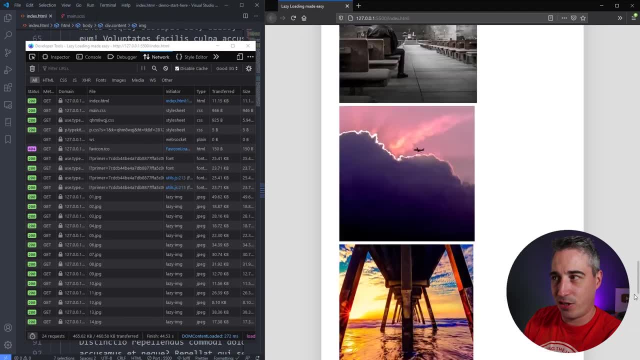 we're going to get to some text in a second and then, and then, as I approach the rest of my images, suddenly those ones all load in as well. And then, when you get those other images that are right there, cool right, 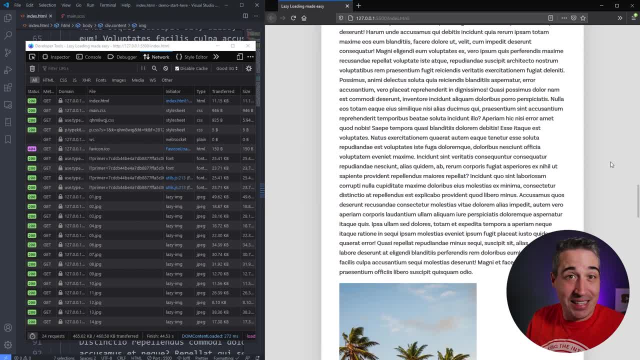 So we're only loading the images in as we need them, And that's what lazy loading is. So if you're on a slow internet connection, you're on a mobile device. it's websites loading slowly, whether it's a bad wifi connection or you don't have great. 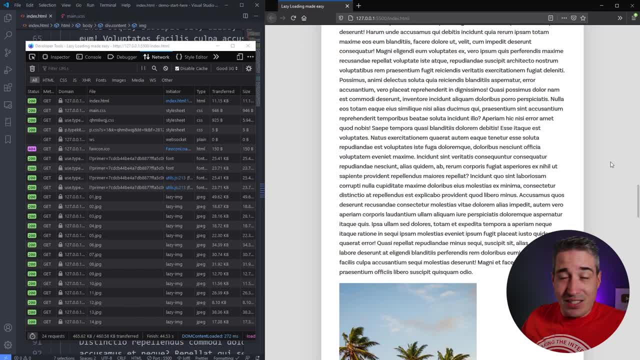 um, you know you are on 3g, for whatever reason. this could save you a lot of data, because if you're not scrolling, you're just clicking to the next thing. That's really cool. Or if you are scrolling, it's only loading them in as they need them. 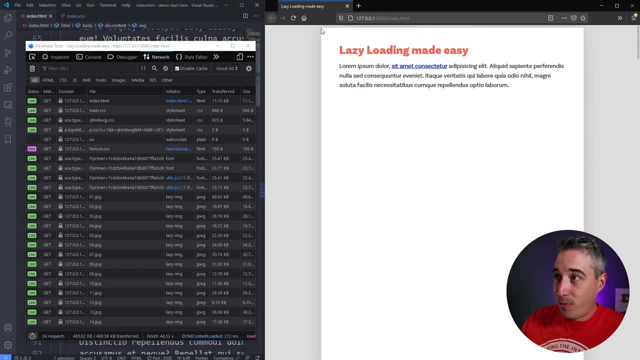 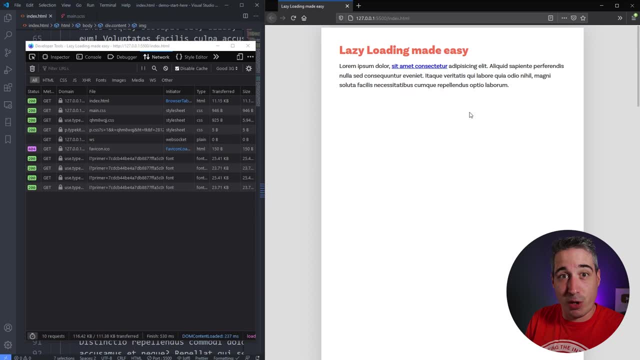 So right away there's a huge performance boost And, as we saw from the very beginning, the initial page load much, much, much faster because there's a lot less things that need to be loaded in for the page to be fully rendered. 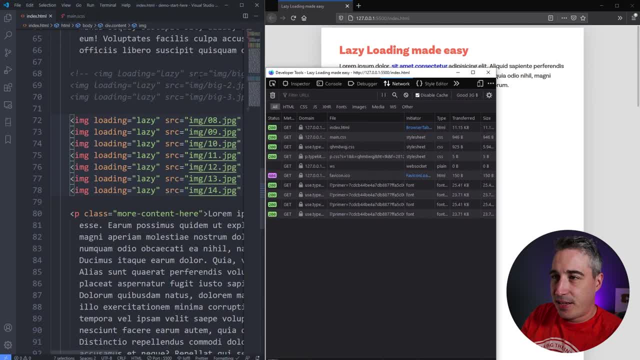 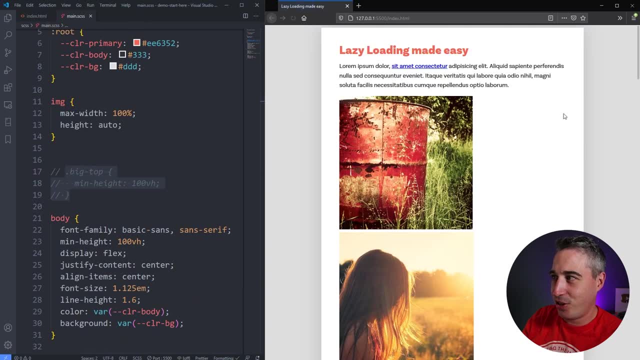 So that's really, really cool. Now, uh, one thing, just really fast. let's just say I'm going to go to my CSS here for one second. I made this big top area where I did a hundred VH because I wanted my images to be off screen at the. 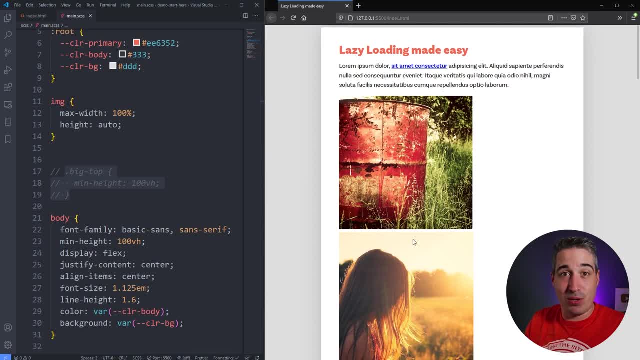 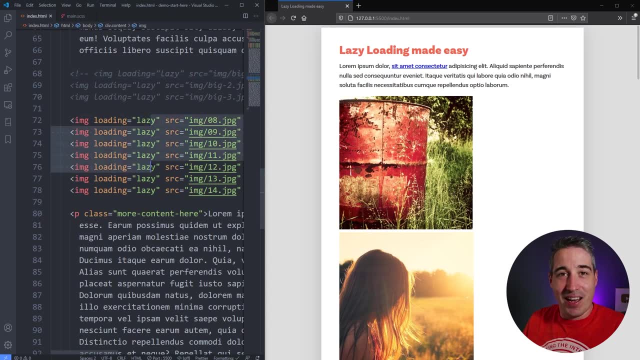 beginning. It is recommended that if the images are visible at the uh when the page loads, that you don't actually put a loading equals lazy on there. we don't want this to load in a lazily, We want it to be there right when the page loads. 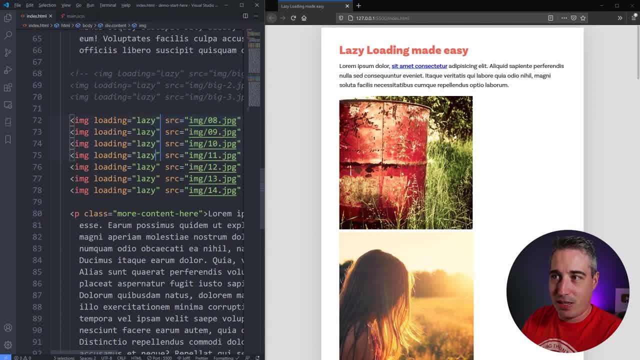 So I could come in on, say, the first four images here, just because I want to be safe and you know, you don't know screen sizes and stuff, and I could leave it off on those ones. Um, and then I could leave it on for anything that would. 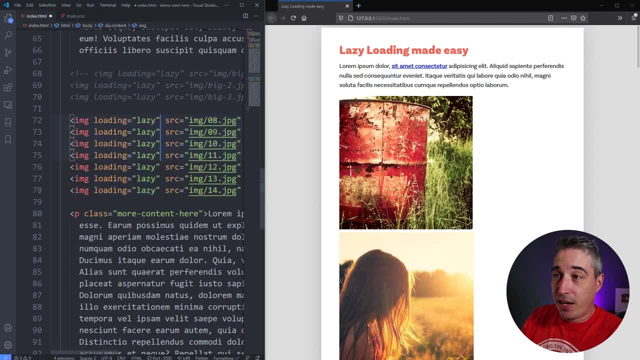 be lower down on the page, And that would be completely fine. Uh, another choice that you do have is you could actually come in and put eager on these. Um, eager is the same behavior as if it wasn't there, though. Um. 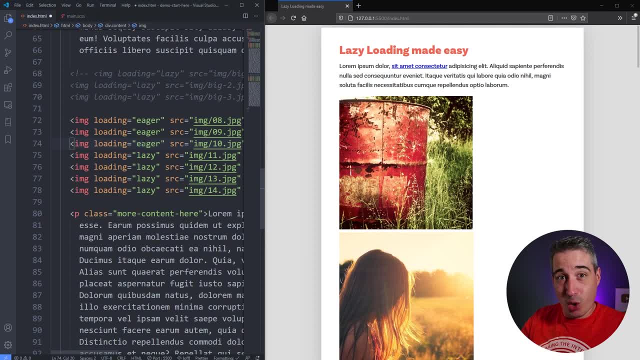 so eager saying no matter what, even if this is could be like an image all the way down at the bottom loaded in, even if I, even if it's not close to being in the viewport. Um, now, we don't have to include this because it is the. 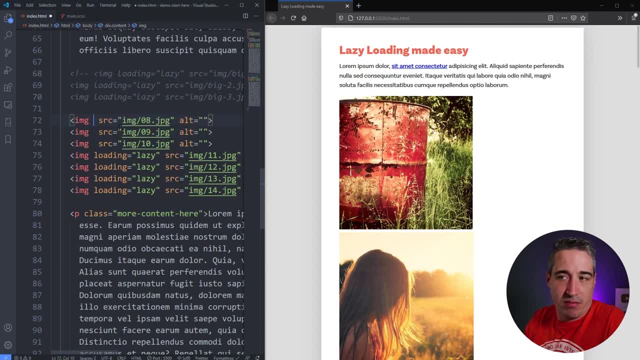 default behavior. So if you just leave that off, then you're not changing anything, or not changing too much there. Um, so that is an option as well, right there? Um, but we can include the lazy. It's generally not something you'd want to do if it's. 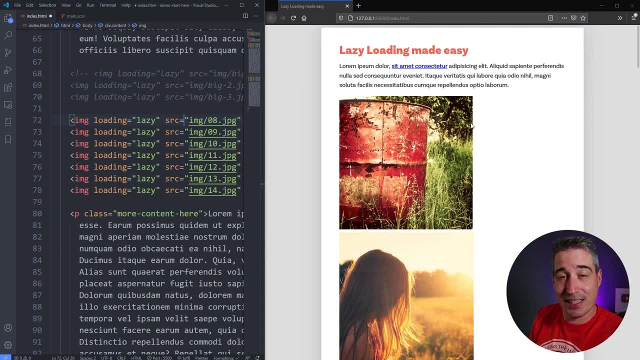 something that is above the fold, But if it's anything where a user would scroll to see it, then you'd want to include your loading equals. lazy Now to show you. I think one of the issues that people do have with it is these jumps that happen. 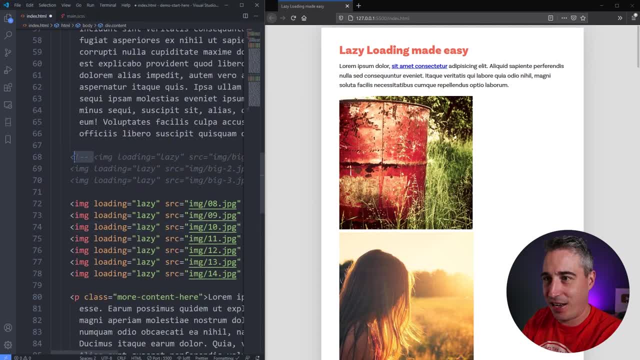 So I do want to show you what I'm talking about, And I have these extra images that I have right here. Uh, so let me just see if I can on comment those and let's take these ones out, because we're gonna have too. 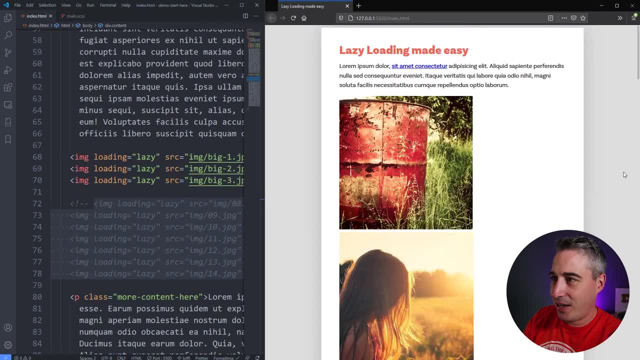 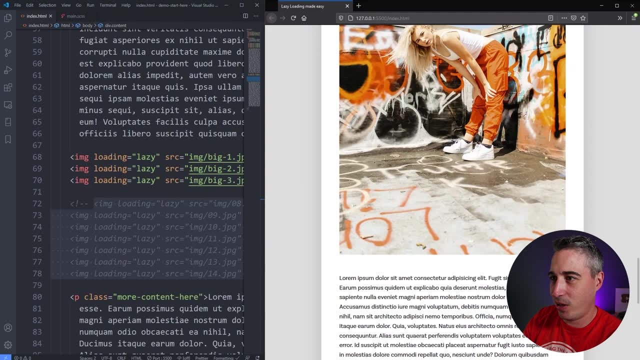 many images, If not, and we'll hit save, And if I come down far enough, we'll find some big images right here. There's one and there's more, but this one it's loading in slowly. Oh boom, there's another one. 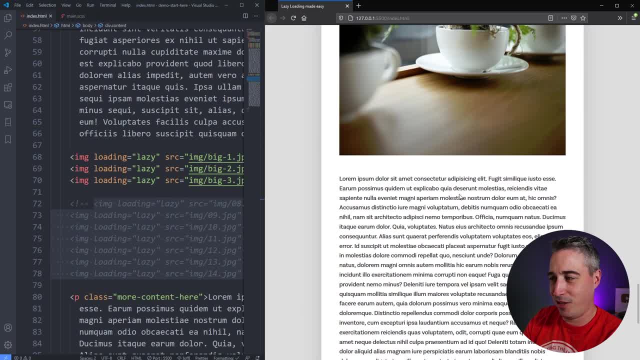 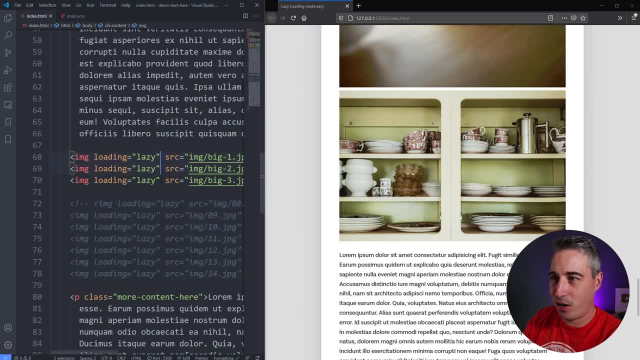 And then come on, slowly but surely. These are big images. There are each over a meg, and we're on a slow internet connection. and boom, there's the next one, And actually I had lazy loading on these already, So let's just take that off. 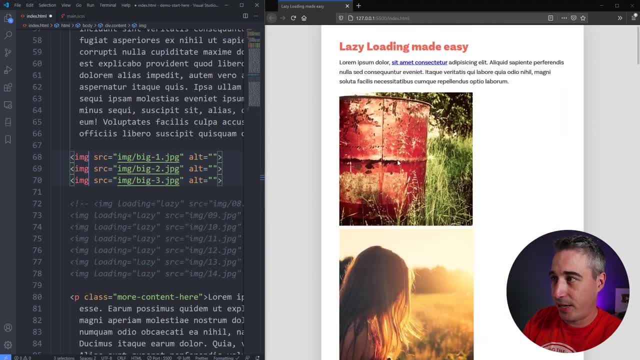 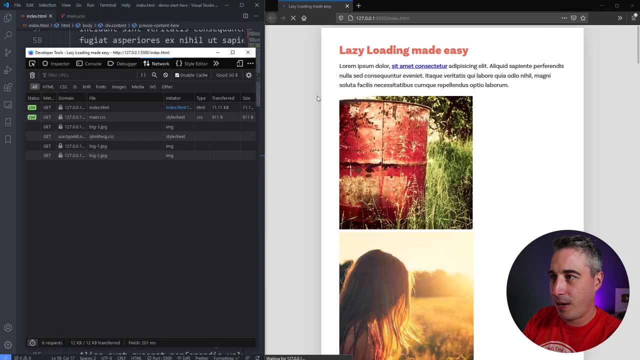 And just to show you- um, it is an exaggeration what I'm doing in this case, but I'm going to come all the way up. Uh, let's bring this guy over here. Um, and when the page reloads. 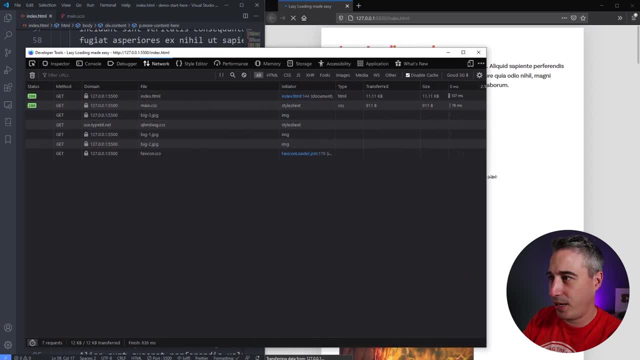 you can see the big one is coming In and actually, can we get that cascading the waterfall you're going to see? uh, we're sort of stuck right now, Actually, um, it's taking so long for these images to come in. 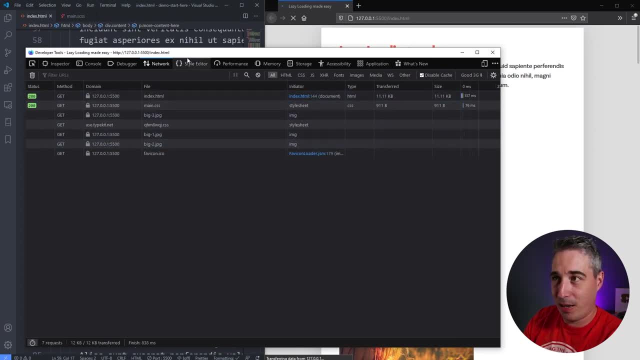 It is actually caused a bit of a problem, but a bit of a backlog. My image number three hasn't come in yet. You can see the page is still going. Oh boom, there we go. Big threes finally come in Um. 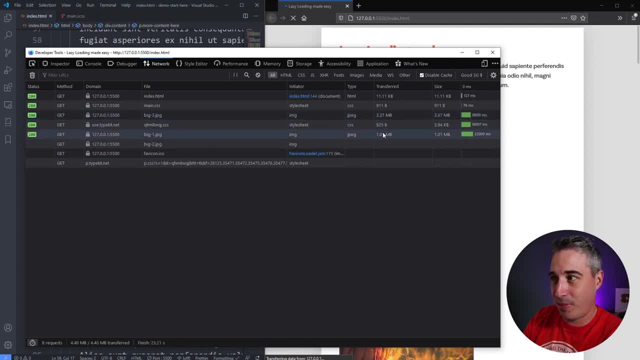 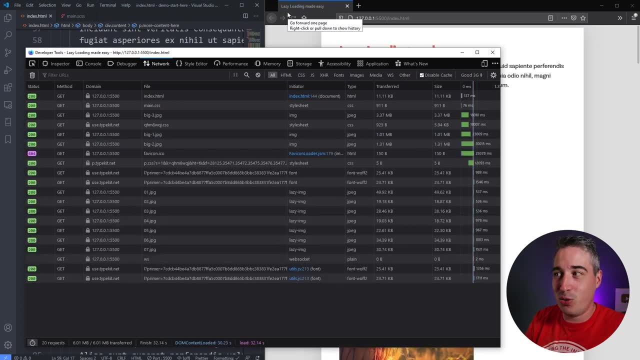 this is really slowing my site down with these big images. That one's three megs, This one's one meg. So this is like putting the brakes. My page is still loading right now. It's really putting the brakes on Now. don't use lazy loading. 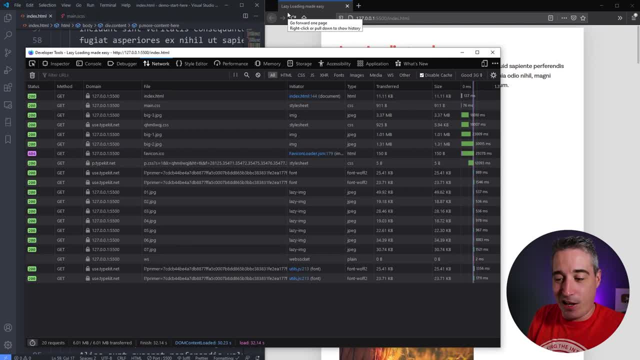 Lazy loading to get around images like this. please don't go. Oh, I can now put a three megabyte image in my website. That's not at all what I'm saying. I just want to show you one of the problems that lazy loading can cause and the 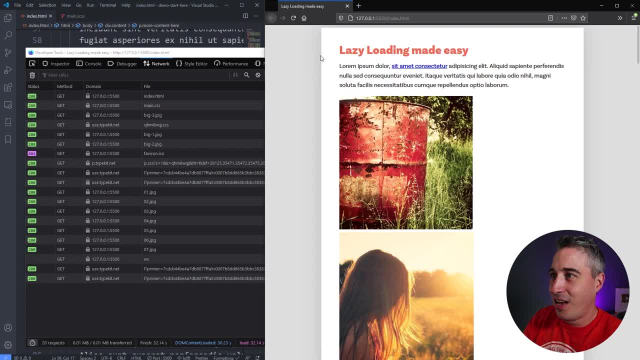 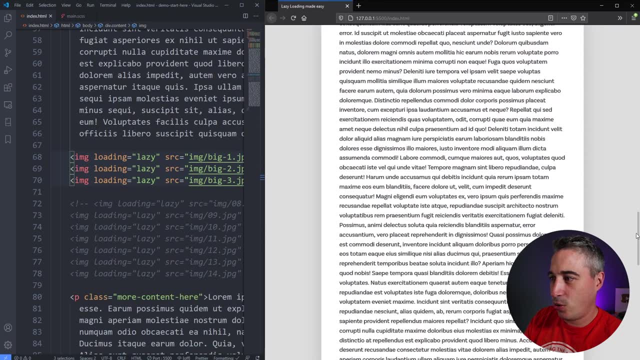 fix that you can use for it. So that's why I brought these huge images in, Um. so here let's add the uh, the lazy loading back in when I scroll down, though what's going to happen is I'm going to get to some text, and then boom. 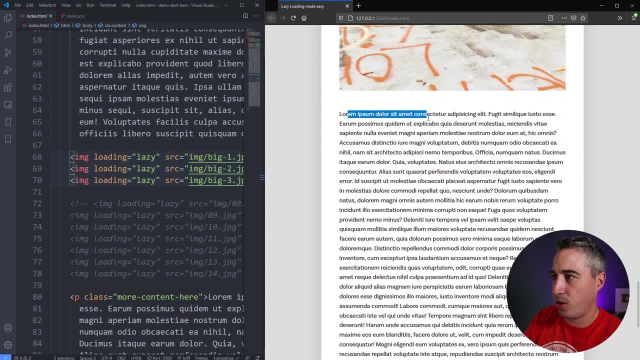 Oh, it's gone, My text. Okay, that's okay. Let's start reading this: Duh, duh, duh, Laura, Mipsome, consent, or at it. Oh, where'd my content go? Okay, Oh. 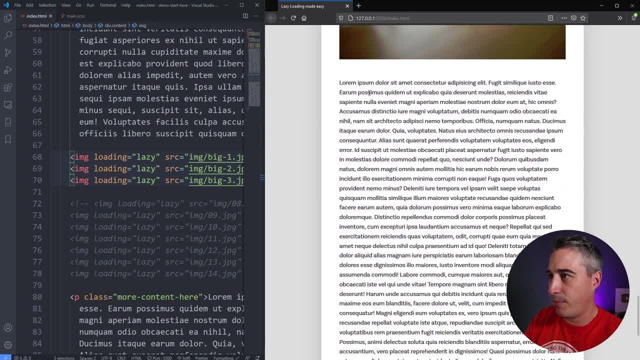 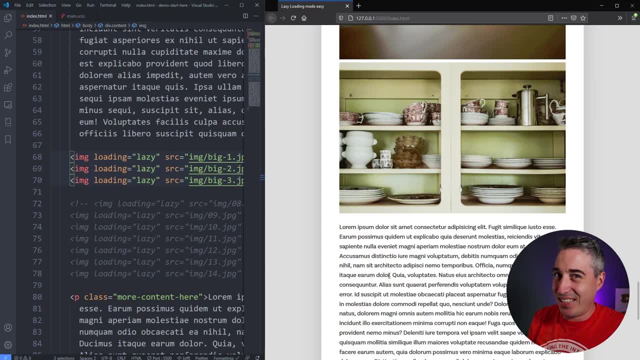 there it is Again. food gets into the dumb essay. Your Ram possum, I can't read Latin, but Oh, my content just shifted again. I'm sure you've been on a phone or something like that's happening. It's usually ads that are the culprit here, where, as the ad loads in, 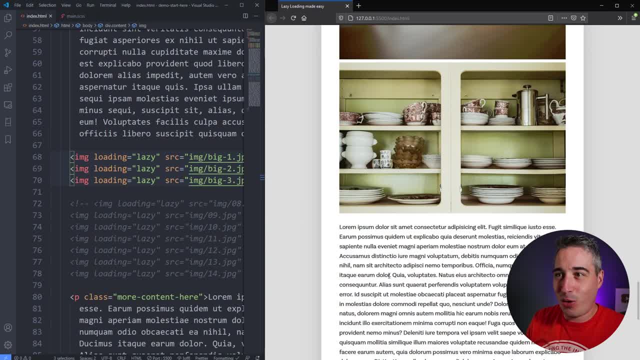 uh, all of a sudden, the content on your page is shifting around. One really cool thing with lazy loading is you can also do this on iframes as well, So that could be useful for ads. Um, and another thing you can do with iframes as well as images is you can give 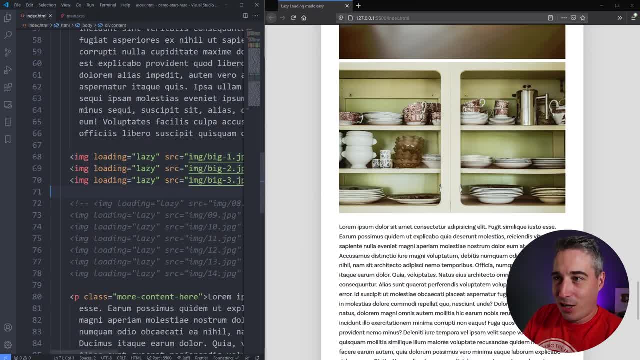 them which, which, which, which, which width and height attributes. So I would strongly encourage doing that on any images you have, Um, so I'm going to speed this up, just as I bring a width and a height on here. 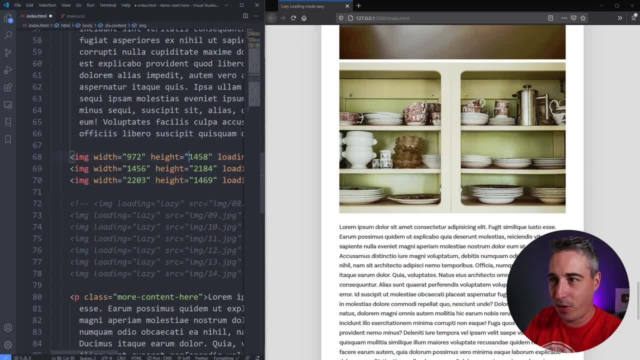 Okay, so there we go. You can see, I now have my width and my height on all three of these images, And so let's uh here, come back up to the top and hit refresh, and all our content should start coming in. 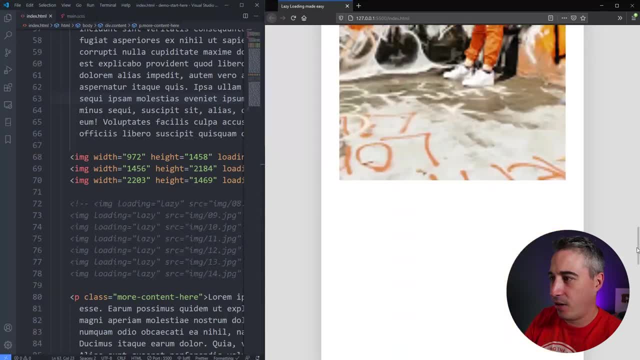 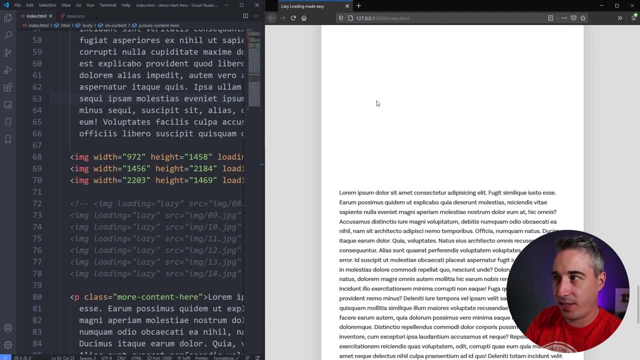 But the advantage, now that I've given it a width and a height, is when I get here, you can see there's actually these big blank spaces. So even though the images haven't finished loading in yet, there's gonna be no jumping content. 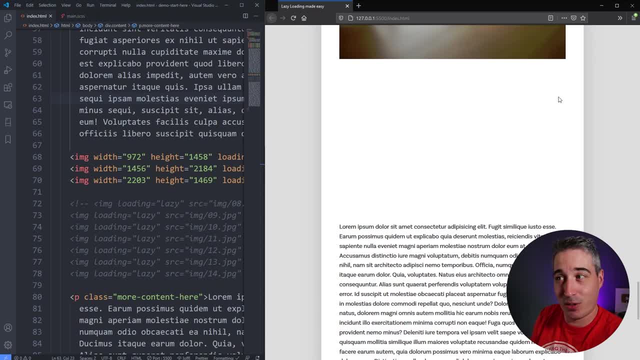 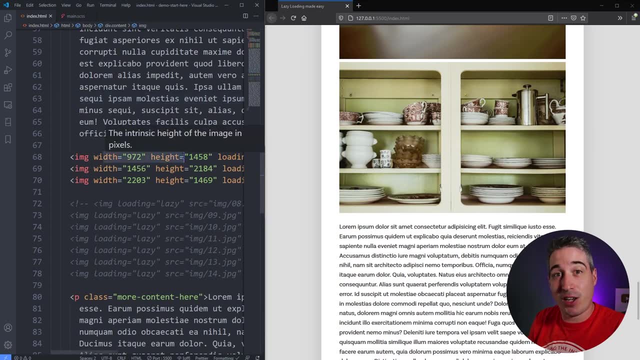 When, when that image comes in, there's a placeholder here. Now it's completely blank placeholder or it's holding that space because the browser knows that image is coming. So by assigning the width and the height on here, it's automatically just going to work and you're not going to get weird jumps. 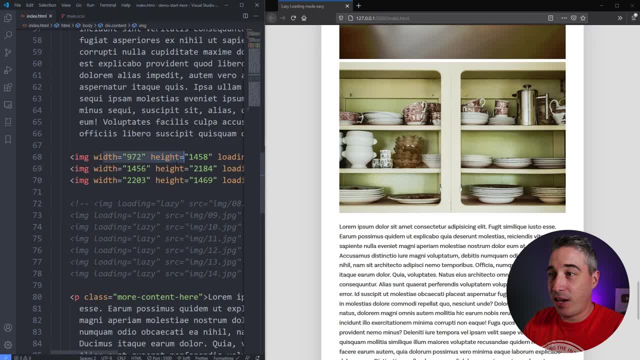 in content. This is the same for iframes as well. Um, and another advantage and cool thing with this now actually is: Firefox was the first one to do this, Chrome has implemented it and Safari's in the process of implementing um, another feature that comes with your width and your height and what that is. 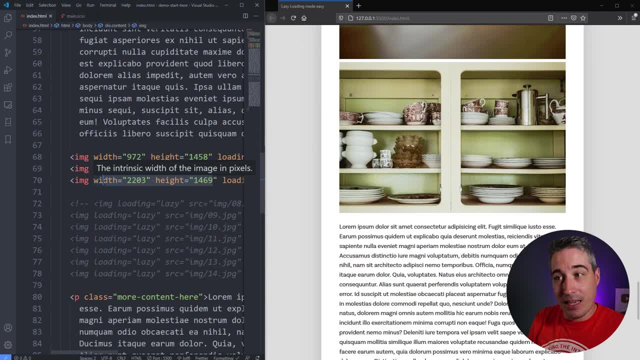 is, if you assign a width and a height, the aspect ratio of the image is automatically calculated by the browser. So when we resize things with CSS cause these are massive like. do not have images that are this big in general on your site unless you. 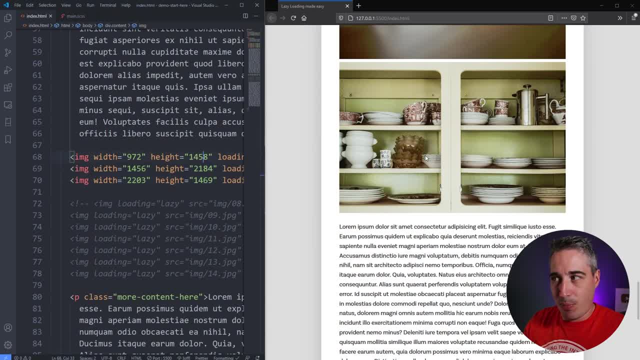 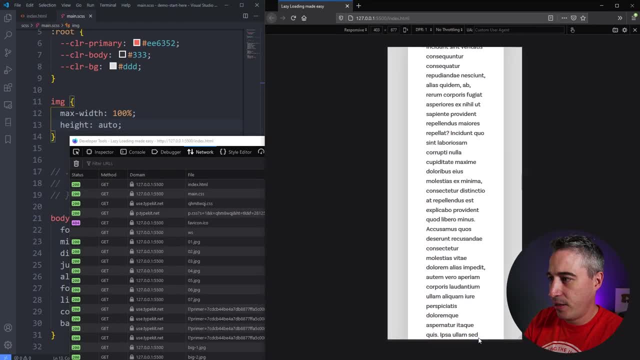 have a really good reason. Um, but these are huge. They're not that big on my screen right now because I'm using my max width and my height auto to resize them. Um, if I resize this, my images are resizing with my browser window right here. 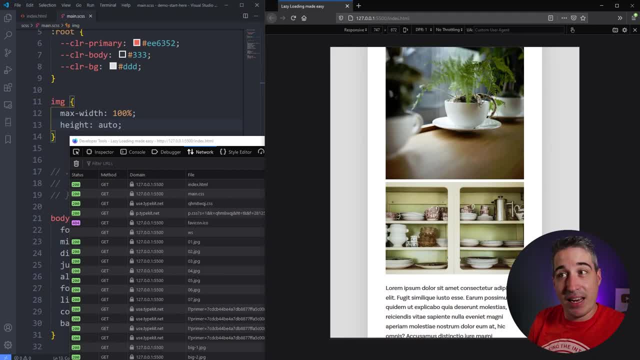 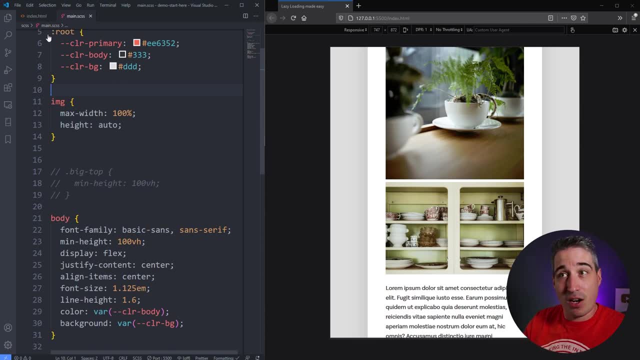 the viewport grows and shrinks, They has to be resized, And when images were resized, it actually used to cause things to be repainted a little bit. The browser had to recalculate everything If you have a width and a height assigned as attributes. 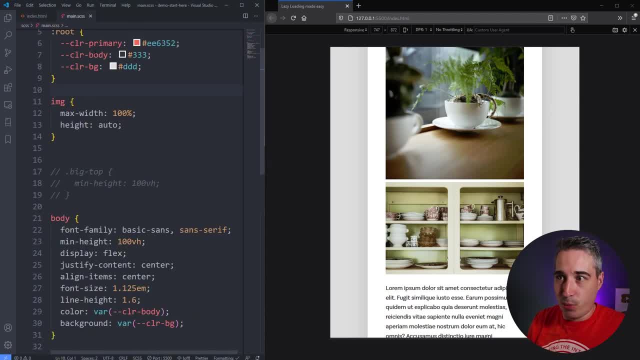 now. it actually speeds everything up and makes everything a lot smoother. Uh, when you have something like this that's on there now, you do have to make sure you don't only have a max width, because if your height is not set to auto, they are going to stretch because it's going to keep the height attribute. that 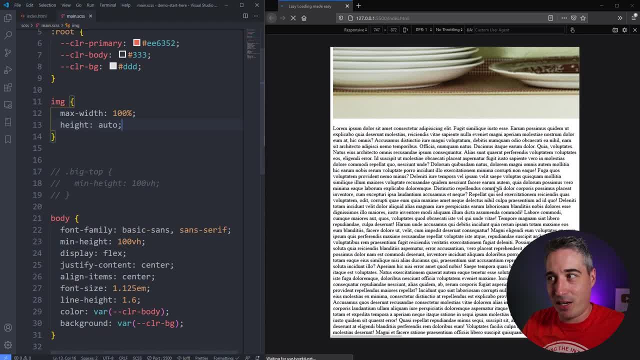 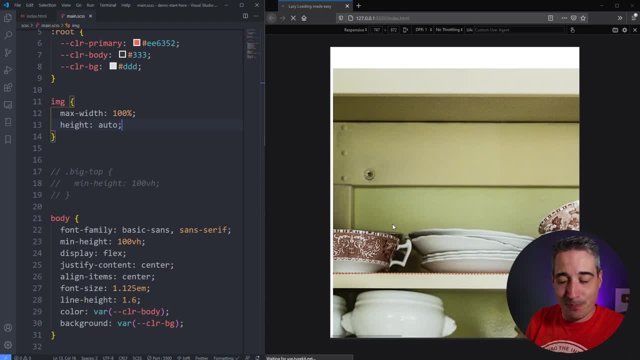 you put on there. So you will have to put max width a hundred percent and your height of auto to actually get everything to work and not to be broken. But overall it can work really, really well. Now there are more advantages to doing the lazy loading here with this as well. 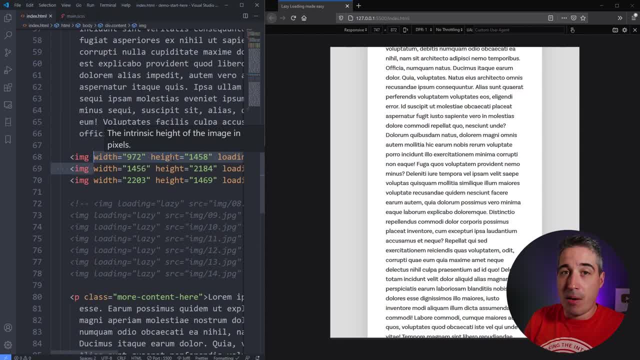 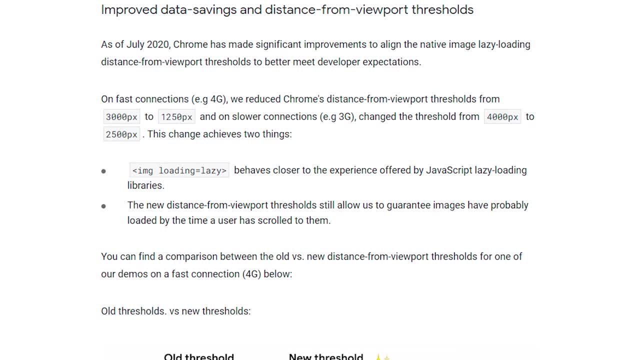 Now, every browser technically can implement it a little bit differently, but the Google, for example, they actually show that if something's on a 4g network, images will load in when there are 1,250 pixels away from the viewport, But if they're on a slower connection. 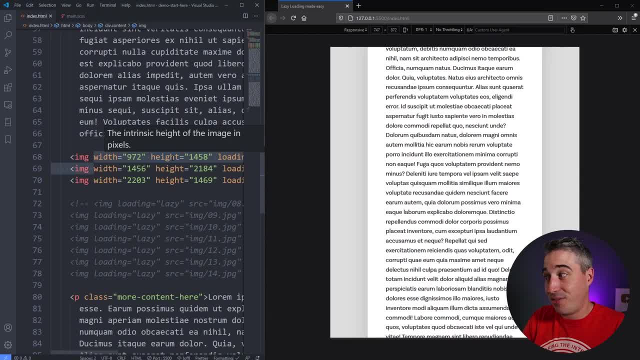 like a 3d 3g connection and to start loading them in when they're 2,500 pixels away instead. So a JavaScript. it was always just based on intersection observers or scroll event listeners, And as an image got closer it didn't know about the connection speeds and other things like that. 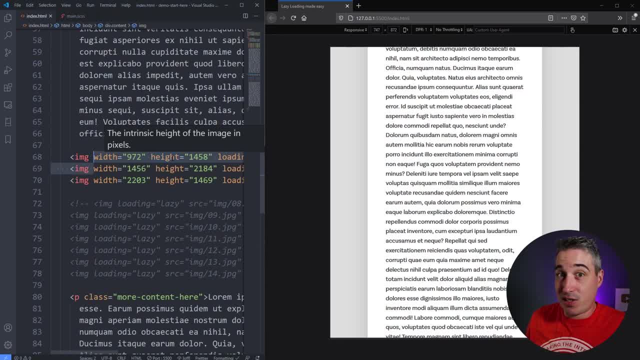 So the nice advantage here is the browser can figure that out. It goes. Oh, it's a slow connection, I'm going to load it in earlier. Oh, it's a really fast connection. I can load it in just as soon as that image is coming into the viewport. 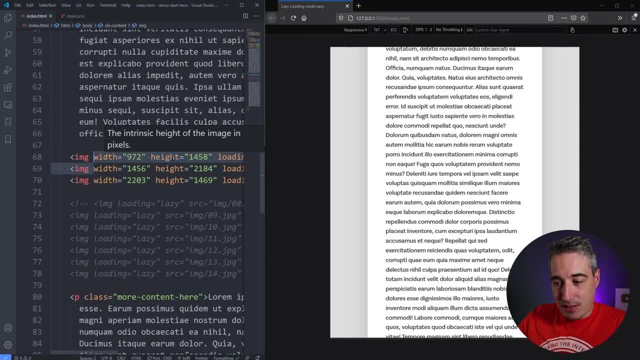 Another really nice thing with lazy loading images like this is even it's right now. the browser support is pretty good. It's not perfect, but it's coming along. It's in Firefox, Chrome and then Safari. It is behind a flag. 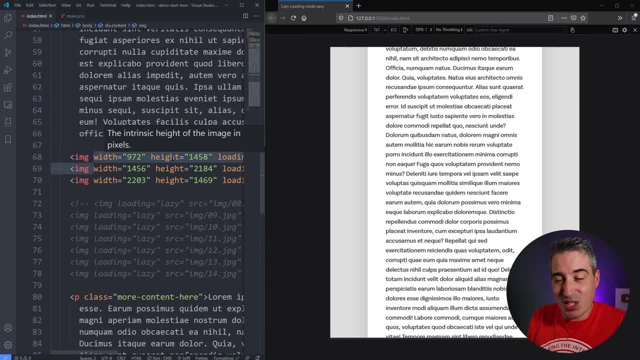 So so it should be coming pretty soon. But the nice thing with this is is, if it doesn't work, your image is still going to load, right. So it's not that big of a deal. You could even if you wanted to rate some JavaScript. 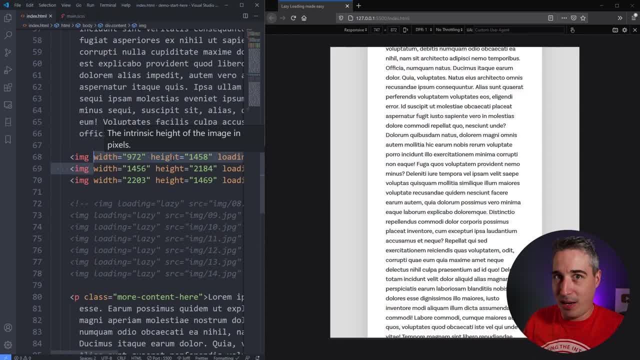 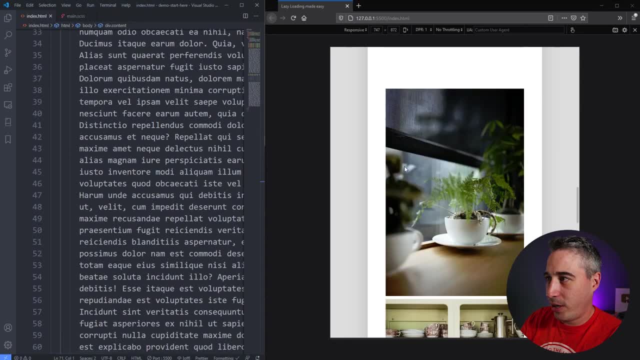 So if it doesn't work, then you could bring in your own implementation of it or something like that, But you do not need to do that. And another thing you can do as well: let's go all the way up to the top here. 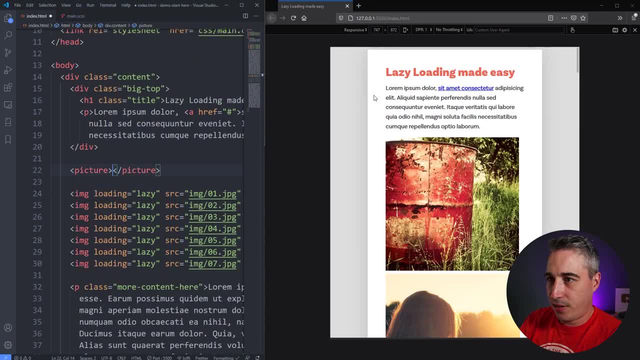 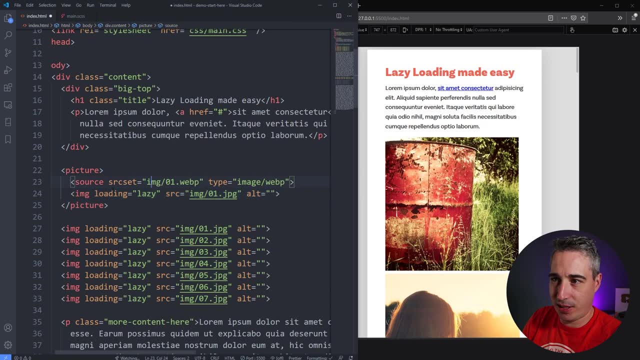 Just for one last image. Let's say you have a picture element and here we go, So it's done. Let me just bring it out a little bit So you can see. here I have a picture element that's bringing in a web P and the default is a. 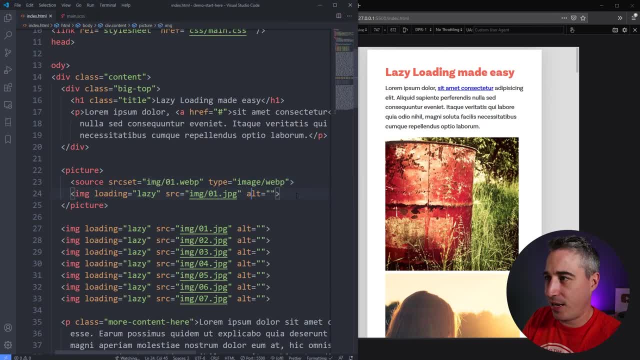 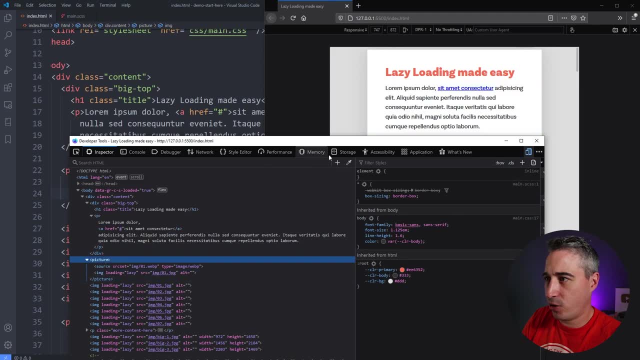 regular image with my fallback pretty much here, And so if I hit save on that it should load in my image at the top, And if I go and take a look at that image itself so you can see it's right there. Let's go to my network again. 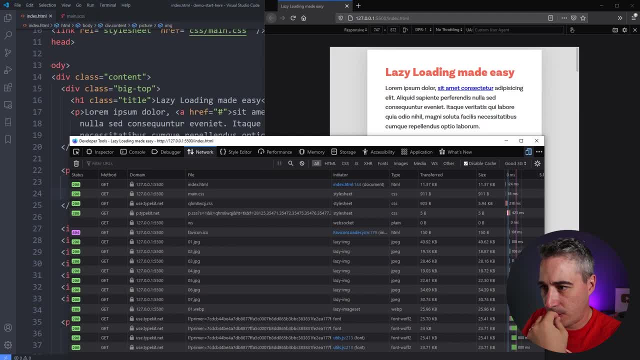 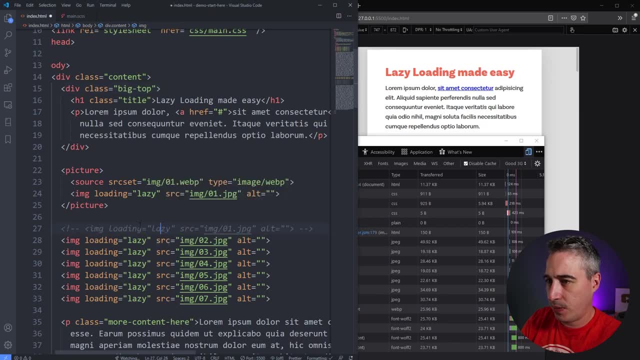 actually- And you can see it has loaded in my web P image right there. So actually, if I turn off this one and we go take a look, we shouldn't see a zero one anywhere except for the web P. So even though I have loaded in my image with this, 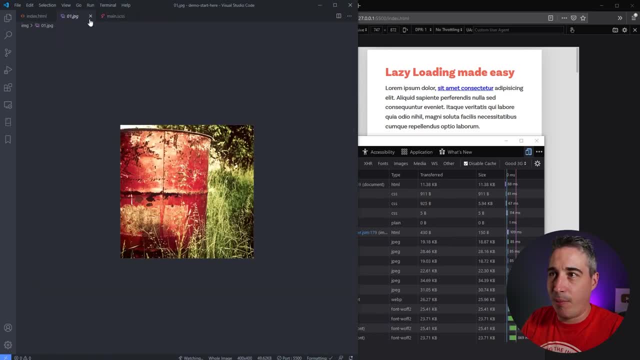 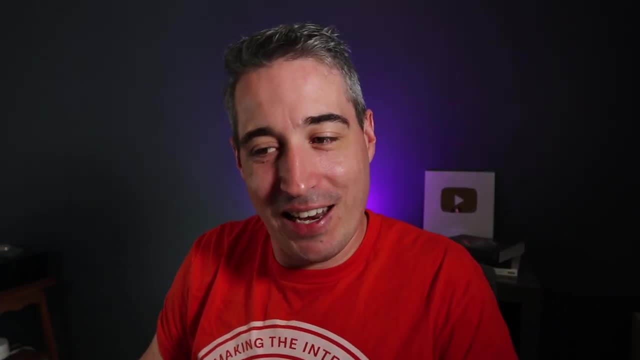 this is the fallback. It's going to use this source instead, And using things like web P is another really nice way to optimize your websites. If you haven't dove into the world of web P and other things like that, I have a full series on optimizing images for the web. 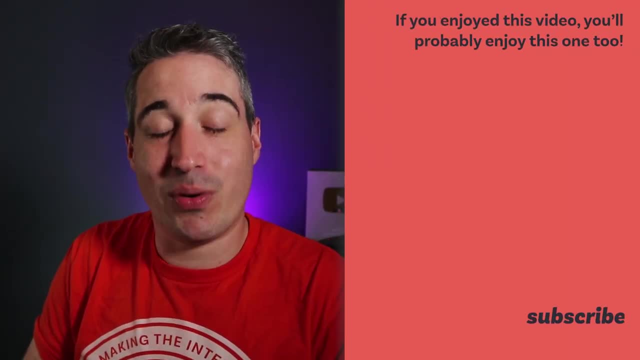 but maybe you'd be interested in you should be able to click the link on there right now. I want to say a really big thank you to Skillshare for sponsoring this video. If you are interested in checking out their deal for two free months. 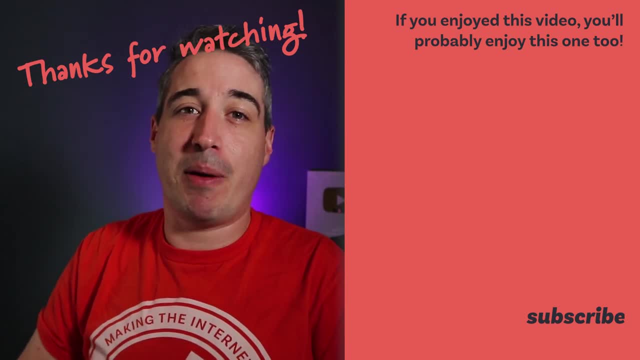 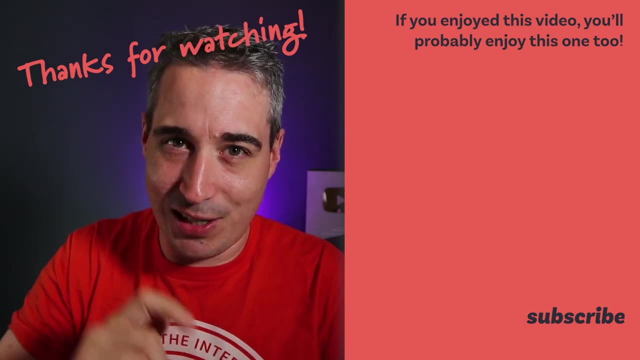 go in. click that link down in the description below. a massive thank you to my patrons for helping support me every single month. You guys are absolutely amazing And, of course, until next time. don't forget to make your corner of the internet just a little bit more. awesome.